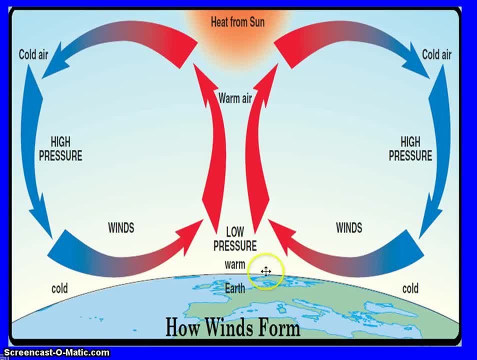 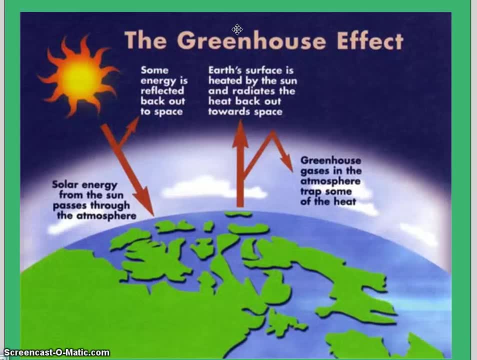 and so that's what creates our winds. so without the sun, there wouldn't be any wind and we wouldn't have any weather actually. Now, another effect of our sun, aside from causing winds, is what it does, and in terms of heating our earth, and you'll notice that it says solar energy from. 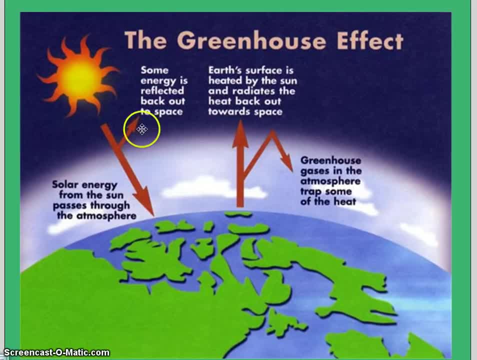 the earth to the earth. So it's a very cold and very hot atmosphere and it's going to cause a lot of heat to pass through our atmosphere. Our atmosphere is going to reflect some of that energy back, but a lot of it actually comes through our atmosphere and that's good for us. 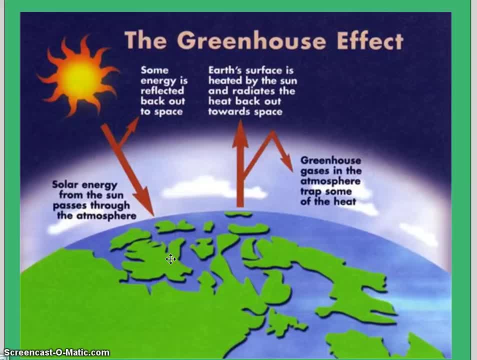 because it keeps our earth nice and warm, as opposed to some of the other planets that lack an atmosphere. They're either super hot or they're very, very cold. Our atmosphere kind of keeps us right in the middle. it keeps us cushioned. You also notice that it says that earth's surface 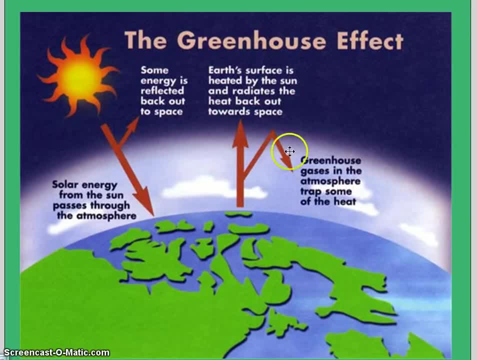 has some heat from the sun and it radiates that back out toward the space. so earth actually loses some of its heat as well. but what keeps some of that heat in is also our atmosphere. and notice, the title of this screen says greenhouse effect. What that is is where the gases in our atmosphere 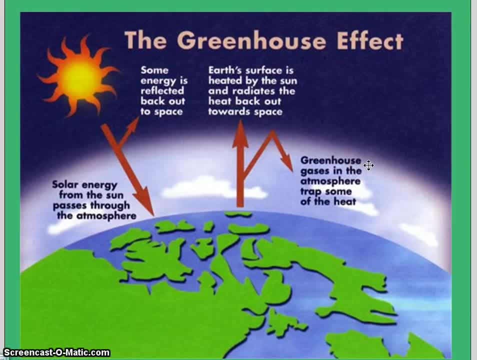 which we call greenhouse gases, like carbon dioxide and water vapor. those greenhouse gases will trap that heat in our atmosphere. It's a very cool thing to do because it keeps us warm. So between the sun giving us that solar energy and the atmosphere trapping some of that energy, it keeps us nice and warm and makes life possible. on 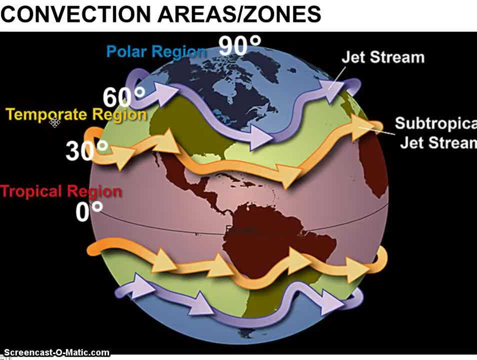 earth. Now, in the first slide we looked at the different angles that the solar radiation hits the earth, and it does change the temperatures of those areas, and so we're going to give those a little bit of a name. These are called conveyor waves, These are convection areas or convection zones, and you'll notice that there are degrees, latitude. 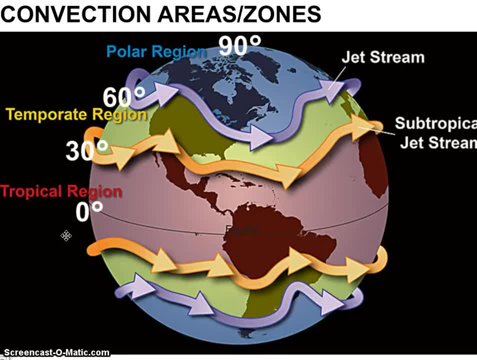 here. so we need to know these ranges for these different heated zones. Well, the hottest zone is, of course, at the equator, and we call this the tropical region, and it extends from zero degrees latitude, which is the equator, to 30 degrees in latitude, and you'll notice that that is true for the northern. 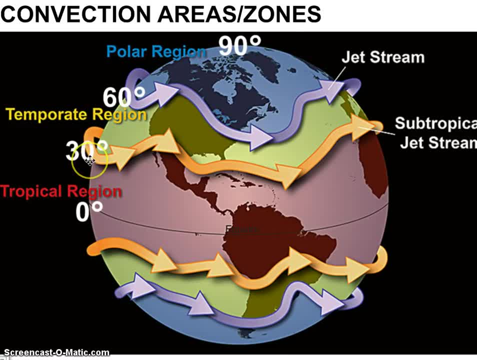 hemisphere. so from zero degrees to 30 degrees north, then that's going to be tropical. zero to 30 degrees south, that's also tropical. but we're just going to be concerned with the northern hemisphere for now. The temperate region is where we live and this is where it's not too hot, not too cold. 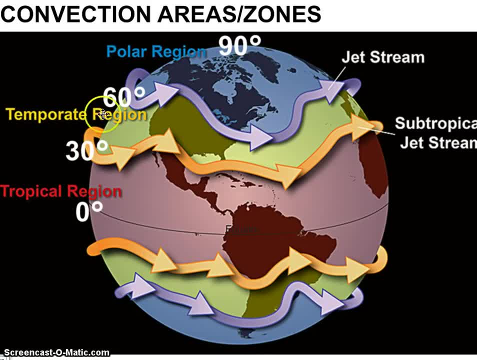 and it extends from the 30 degrees to the 60 degrees north in latitude, so that's the temperate region. and then the coldest region, which is getting the least amount of solar energy year round, is called the polar region, and it extends from 60 degrees north to 90 degrees north. 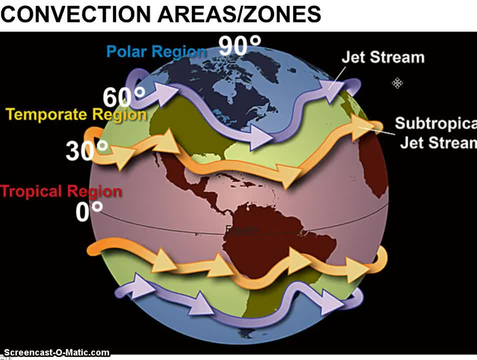 You'll also notice that there's some other types of phenomena on our globe, and that is something called the jet streams, and jet streams are an extremely fast moving ribbon of air that can go maybe a couple of hundred miles an hour, Maybe a hundred miles an hour, maybe a couple hundred miles an hour, that move across our globe. 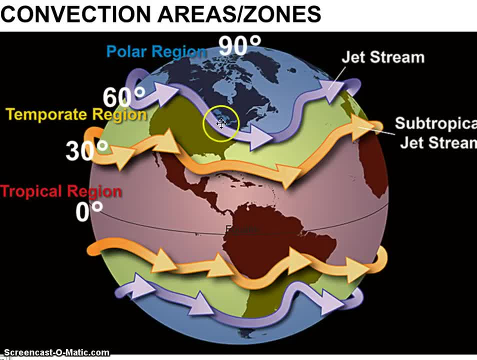 and you'll notice that bordering the northern region of the United States and the southern region of the United States are two different jet streams. The one on our northern border, right between Canada and the US, is called the polar jet stream, and when it dips into our area, it 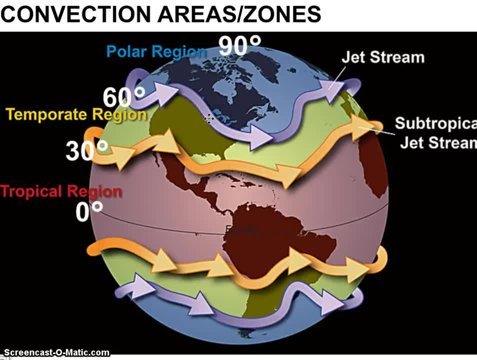 actually brings a lot colder weather, and a lot of that we've been experiencing recently. And then to our south bordering Mexico and the US, is the subtropical jet, and when that moves into our area we tend to have warmer temperatures. Now we know that the sun is responsible for. 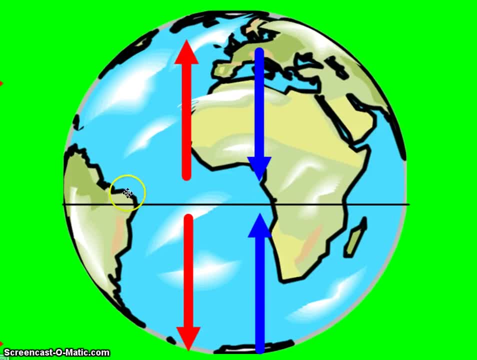 heating up our earth and we had discussed that around the equator that it heats up the most. so we would expect that all of the air that's warm to the equator would rise and go toward the poles and then likewise that cold air at the poles would then just sink straight down to the equator and we 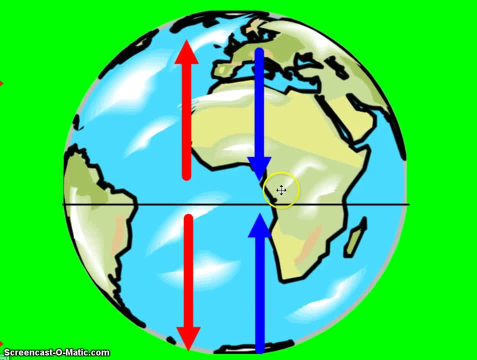 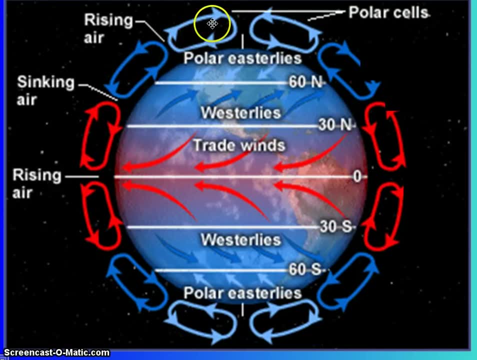 would see one giant convection circle, but in actuality, that's not what happens. In actuality, we actually have several convection cells that extend across our globe, So let's just focus on the northern hemisphere. We have three different convection cells that occur. We have trade winds. 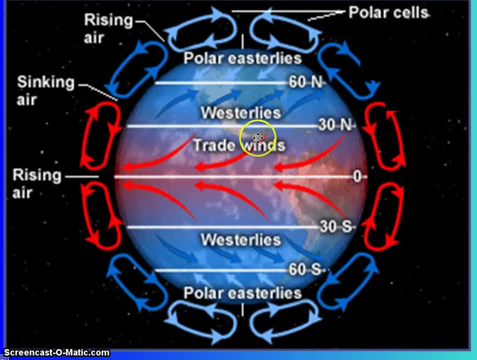 that move from east to west- and we'll talk about why these arrows curve in a separate video- and there's warm air that rises and then cold air that sinks. Even though that these are warm, there's still different degrees of warm. You've got really super hot that rises and then slightly. 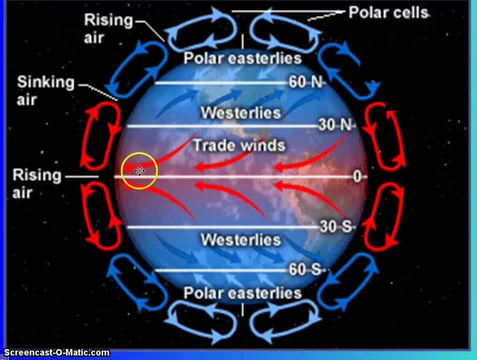 warmer, that's going to sink. So a smaller convection cell You'll also notice in the westerlies- and this is where the United States is And primarily what affects our weather is the westerlies- and we have another convection cell that occurs here: Warm air rises, that cold air sinks, and these are called the westerlies because 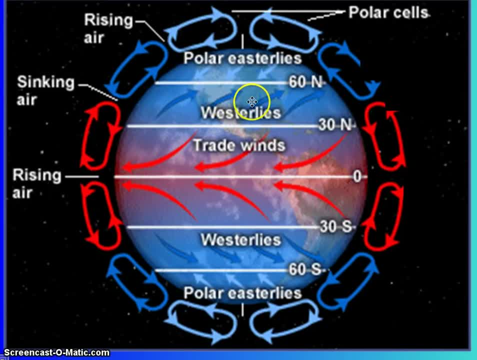 these are winds that blow from the west to the east. This also explains why most of the weather systems, most of the fronts, will move westerly, And that is because these are the winds that we primarily get And, by the way, the jet stream that affects our areas. that's what we call the 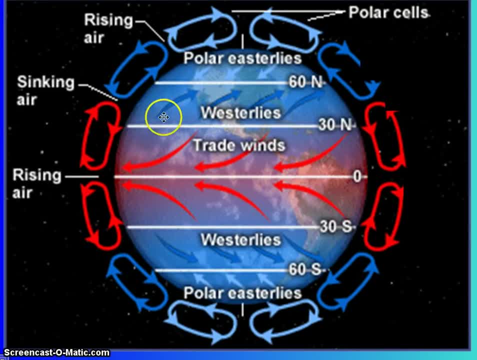 polar jet and the subtropical jet. they move westerly, which kind of pushes our fronts from the west toward the east. So we call these the westerlies where we live, And then we have what's called the polar easterlies. If you'll see these light blue arrows here, they're called easterlies. 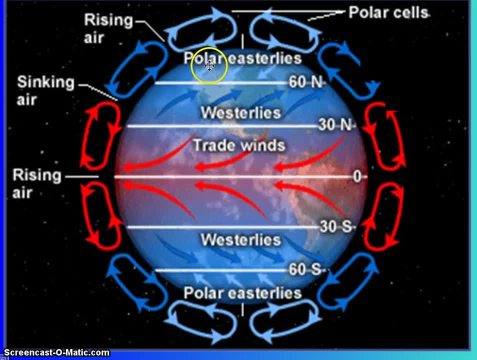 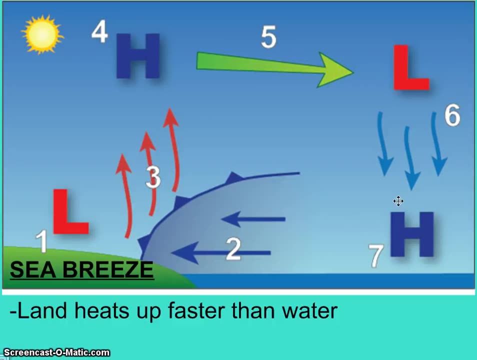 because they're moving from the east and they're super cold, So we call those polar easterlies. So these are what we call the global winds, because these are the winds that affect our globe on a very large scale. And on a small scale, we call these our local winds. We have what's called the sea. 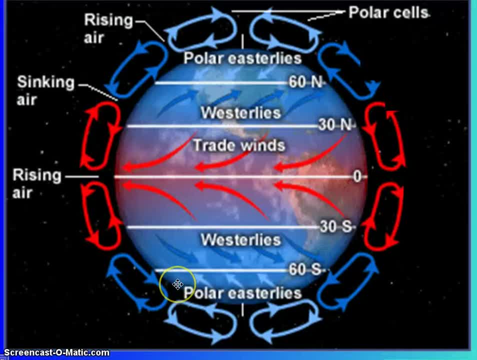 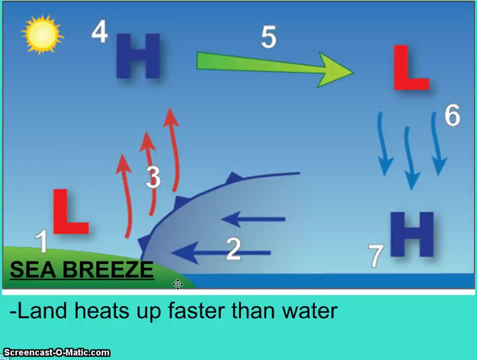 breeze and the land breeze. So these are local and these are global. So there's two different types of winds that affect us. Now, with the sea breeze, that is where we have and, being in Myrtle Beach, we can appreciate this. Sea breezes, they come from the ocean, They come from the sea. 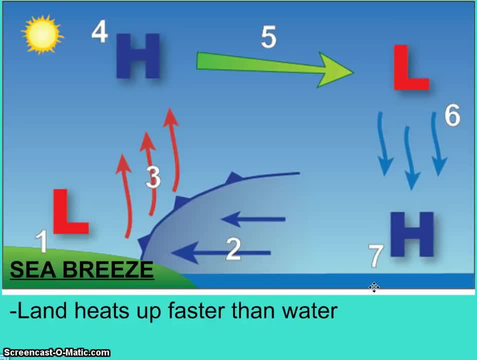 And let's kind of go through the diagram and explain why we have sea breezes. Well, and let's pretend that this is the sand at the beach. It'll help our explanation a little bit. Well, during the daytime, in the summer, the sand heats up a whole lot quicker than does the water, And you know that. 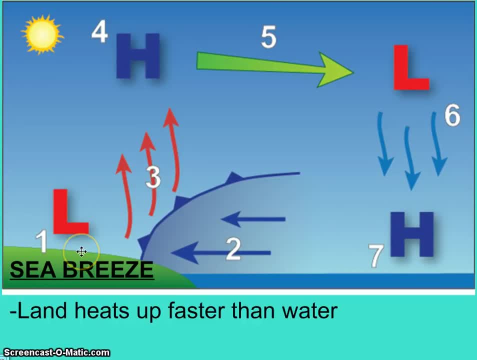 if you've ever forgotten your flip-flops on a summer day, you know that that sand is way hotter than the ocean is. hot that it the sand is hot. it heats the air above it and makes it hot as well and produces an 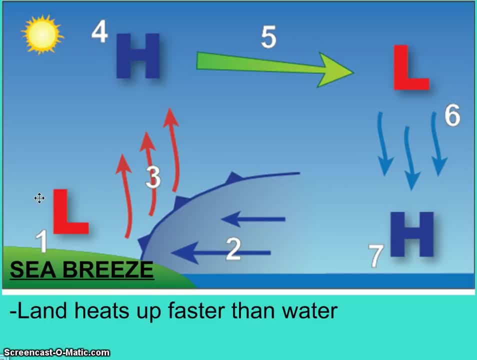 area of low pressure. Remember, low was spelled l-o-w and the w reminds you that lows have warm air. Now let's go over to number two. In number two, we said that this air over, well, the ocean is cooler, which means that the air above it will be cooler, which produces high pressure. 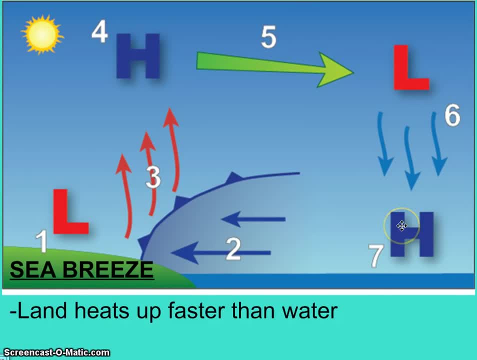 Now, what happens is that this high pressure air is going to move toward- and this is number two here- it's going to move toward an area of low pressure, And what happens, you'll notice, is that a front is created where this cold air is going to win. This cold air is literally going to push. 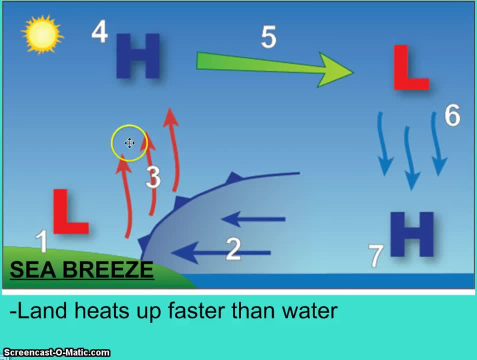 this warm air up with an uppercut. It's going to push it high up into the atmosphere. Now, once it gets there in the atmosphere, that warm air that used to be warm is going to push this warm air up into the atmosphere and it's going to start cooling off because the upper altitudes are cold. 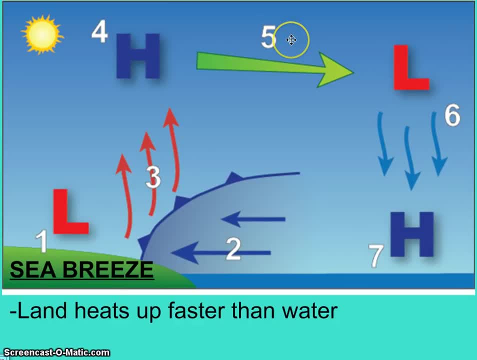 And then, just like we have said before, high pressure always goes toward the low, toward low pressure. So high to low, high to low. And so, at step number five, that high pressure air in the atmosphere is going to move toward low pressure And this air is going to then start sinking and as 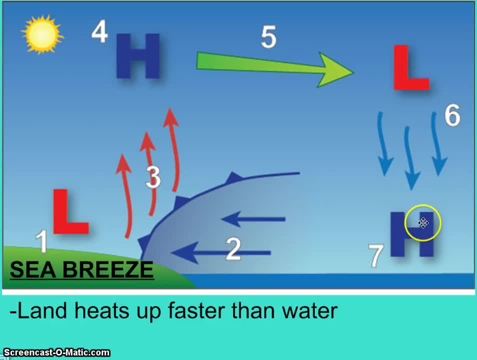 it sinks, it's then going to move toward the land. So this high pressure air that's coming in off the ocean is coming toward the land. So we call it a sea breeze because it's coming from the sea. So just remember, during the day we have a sea breeze Now. 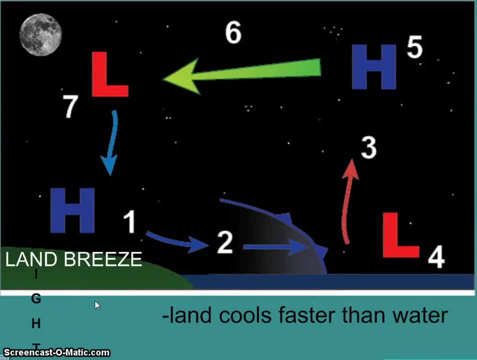 at night we have the exact opposite situation. At night, we have what's called a land breeze, And the way you can remember that land breezes happen at night is to remember the N in land also stands for night. Now this is the sand edge. 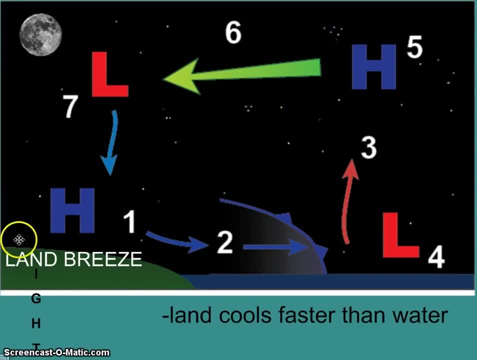 So we're at the beach and we know at night time that that sand is really cool and we don't even need our flip flops. And what happens is- and the reason this happens is because during the day the sand heats up quickly, but at night it also cools down quickly, So it takes all day for the solar energy to warm up. 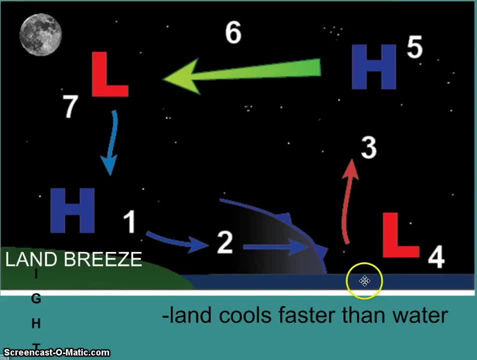 this water so that at night it has that warmth that it gained during the day. So it's retained it. So water takes a lot of time to heat up. So it also takes a long time to cool down. So at night the land is colder than the water. So now what we notice is that high pressure. 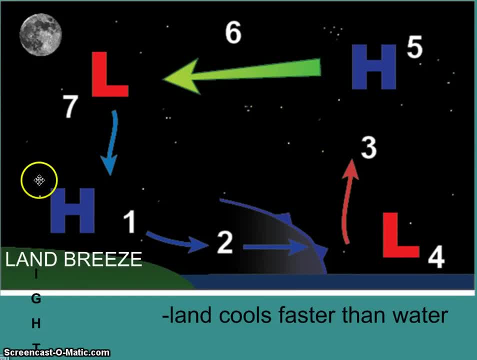 forms over the land because the land is cold, it makes the air cold and that high pressure air is gonna go toward the low. It always goes from high to low, high to low. So this high pressure air is going to have a cold front. It's making a cold front here. 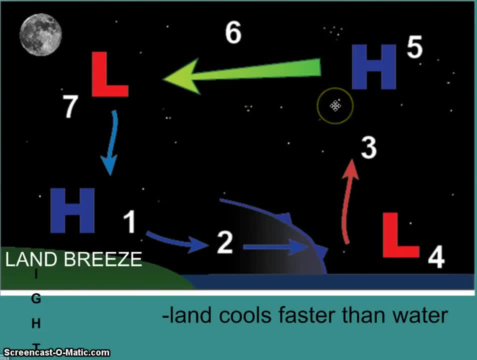 because this cold air is gonna swoop out and push that warm air up, And the air is always gonna go up. So the air around the, that air is going to become colder and what's going to happen is it goes from high to low and 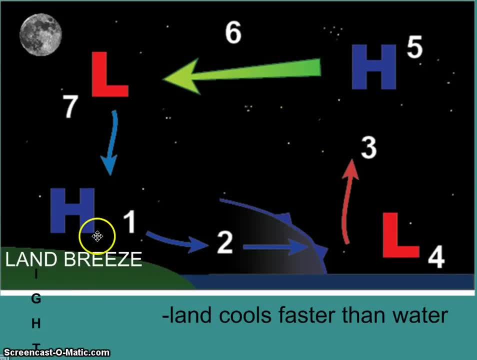 what's going to happen is it's going to sink and then create a convection cell where we have this: cold air is sinking, warm air is rising. now, as this air swoops out from the land toward the ocean, we're going to call this a land breeze, because the breeze is actually coming from the 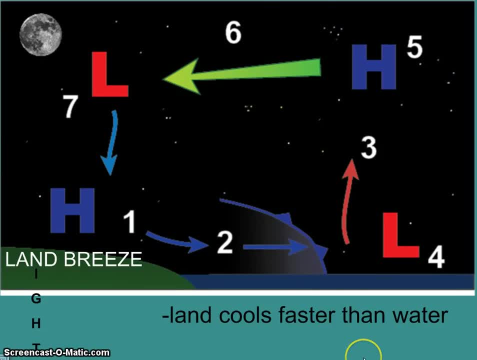 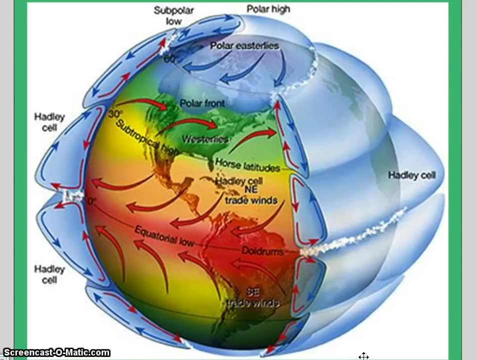 land out over the ocean. so those are some local types of winds that occur. now we want to go back and kind of touch just very quickly on the different convection cells again. again we want to realize that there's not just one giant convection cell. where at the equator, the warm? 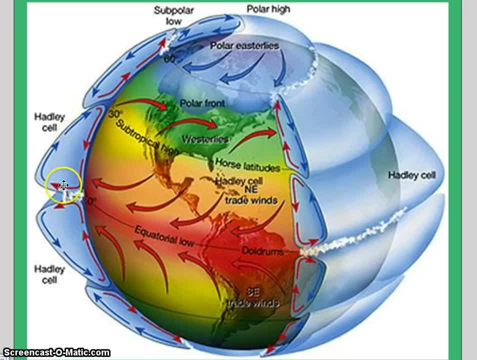 air rises and cold air sinks. we now know that doesn't happen. we have individual convection cells now here. they call them Hadley cells, but we just need to know these are called convection cells. well, the warm air is rising in the atmosphere and the cold 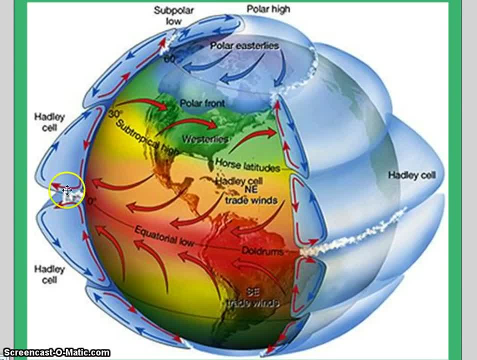 air is sinking, so this is just a different way of looking at it. so warm air rises up. now this is in latitude, it will actually just going straight up in the atmosphere. it rises and then sinks back toward the ground. rises, sinks back toward the ground, all right. another thing. 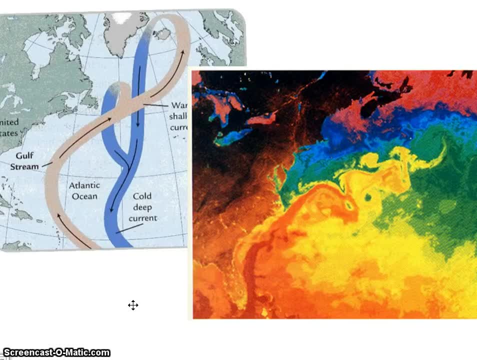 that the Sun affects is not only our winds but also our oceans. so you'll notice that we have the Gulf Stream here, that that water is warm, and so that warm water also will rise and try to go toward the poles, and then, as it is warm at the poles and 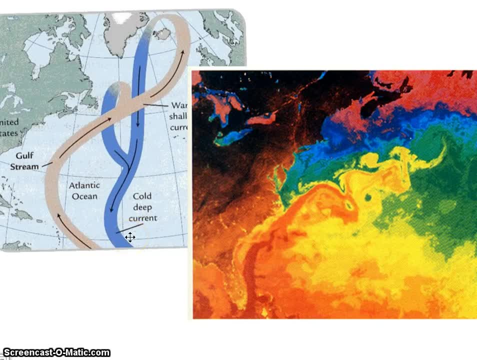 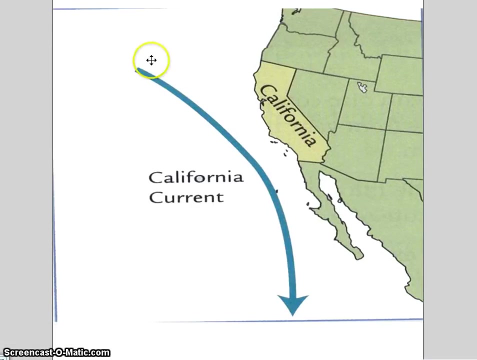 cools off and that cold water will sink. so convection happens with water and with land, and that Gulf Stream actually keeps us quite warm, so that warm water also heats the air. in California they have a different effect. this cold water from the North Pole is sinking here, and so California actually has colder temperatures than 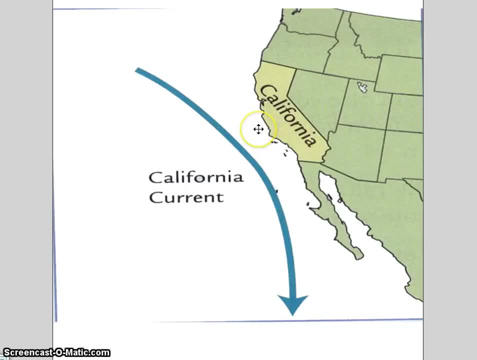 we do in South Carolina. the surfers here in California have to wear wetsuits because that water temperature is so cold because of the California current, whereas our surfers in South Carolina really don't need it because the Gulf Stream keeps us warm. all right, so now we know. 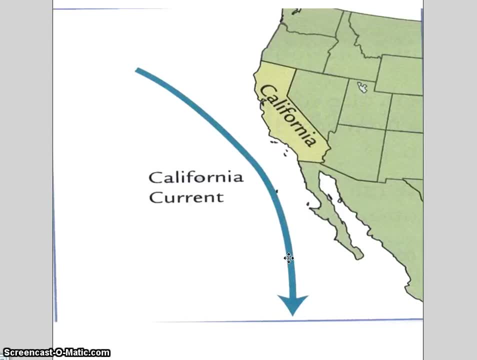 that the Sun affects air on a global scale, on a local scale, and it affects our oceans. all right, so we're going to take a look at the Gulf Stream and we're going to take a look at the.